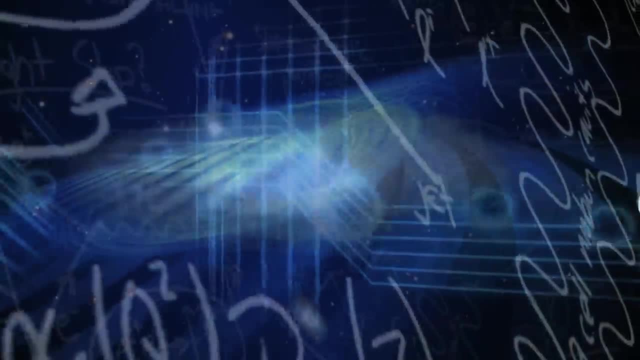 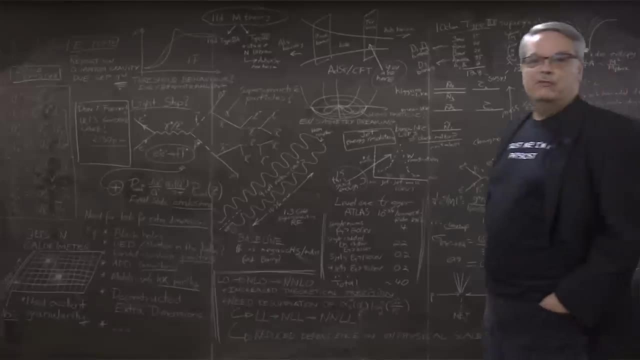 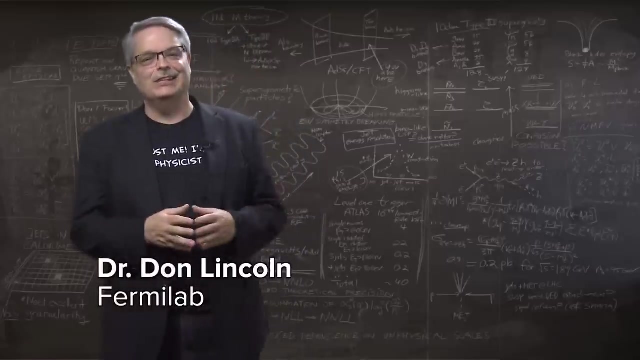 If you're a fan of my videos, you know that I've been on an accelerator kick for the last few, And if you're not a fan, then why the heck not? You should take a look because, well, accelerators are very cool. 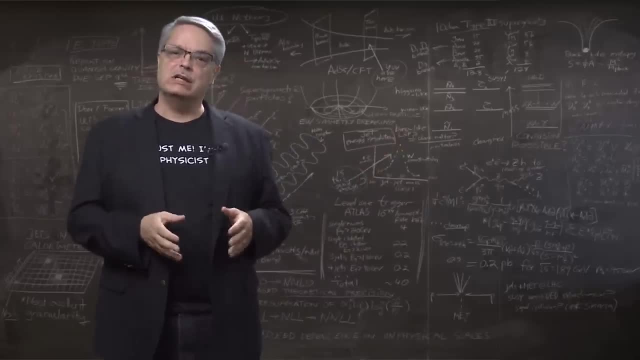 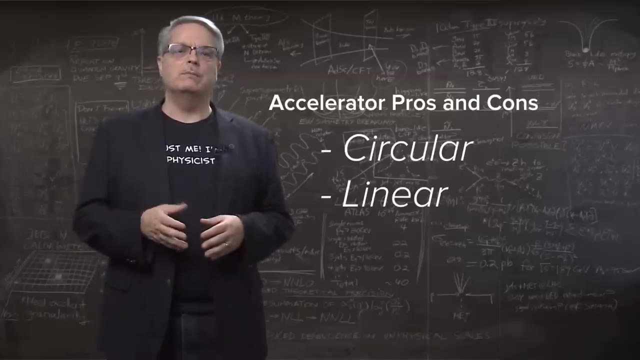 Now, there are lots of different shapes of particle accelerators, but when we're talking about cutting edge research, there are two main ones. One of them is circular and one of them is a straight line. So I thought I'd tell you about the pros and cons of the two. 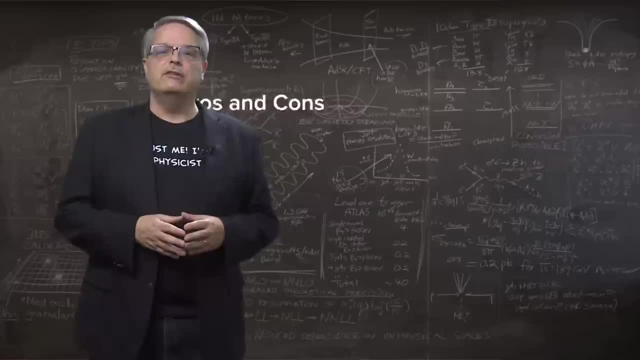 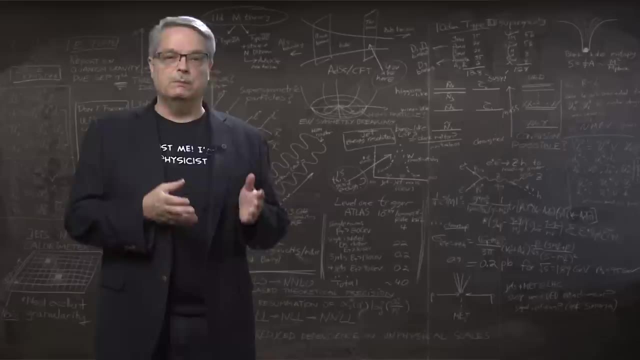 different choices. But first to understand the differences, you need to know how particle accelerators work. The principle is actually really simple. You use an electric field to push a particle with an electrical charge and that particle goes faster. Now the concepts of electric. 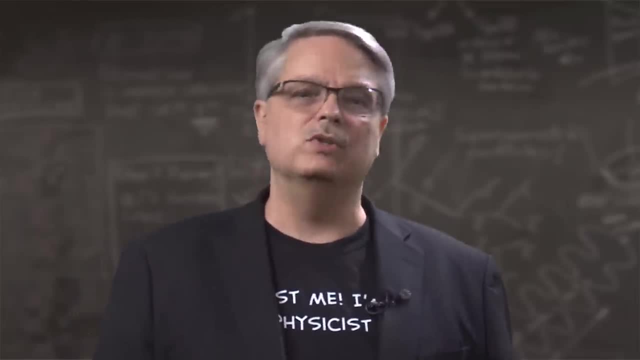 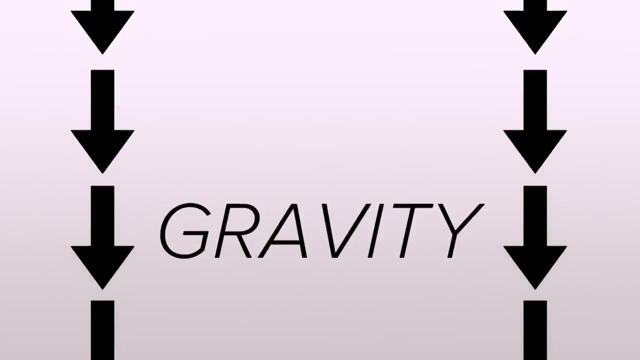 charge and electric fields aren't the most common ideas, so let me use a more familiar situation to help me make my point. Now you all know about gravity and how it works. There's a gravity field that points downwards. That gravity field interacts with objects and have. 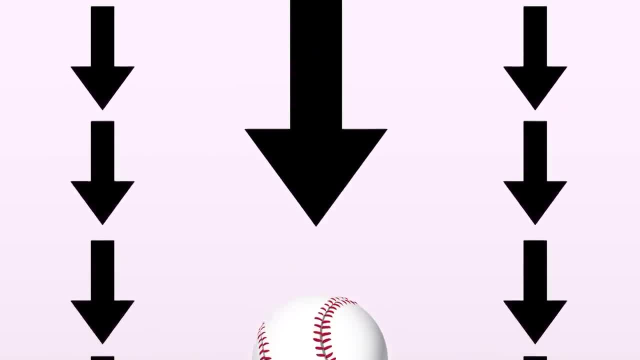 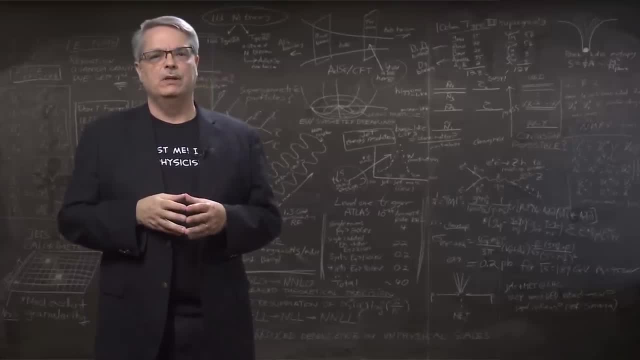 the mass and those objects get pushed downwards. That, by the way, is a techno-geek way to say: things fall when you drop them. But now imagine if you were to change the direction of gravity. We're going to cheat a little bit and pretend there's a cartoon, kind of. 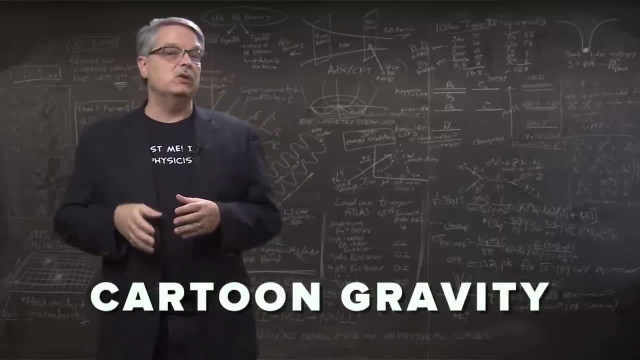 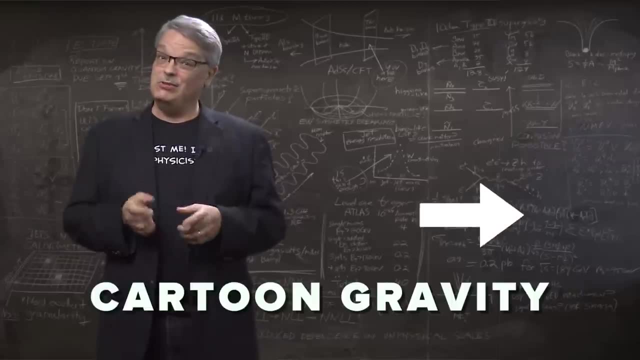 gravity that is a little different than ordinary gravity. I'm going to hold a cartoon ball and see what happens if we have cartoon gravity. point to my left. Maestro, can you point cartoon gravity to the left end? give me a cartoon ball. Oh super. Now if I let the ball go. 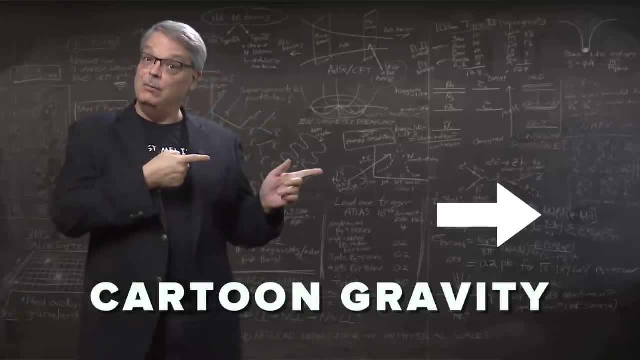 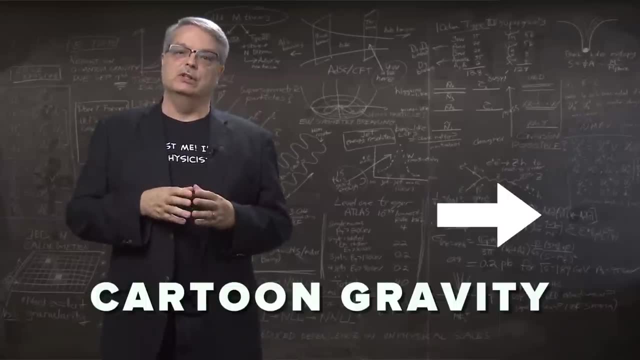 what happens probably won't surprise you. The ball falls to the left. If cartoon gravity points in some other direction, then the ball will fall in that direction. Here let me show you. Maestro, can you pick a direction? Now? I'm going to cover my eyes, Don't tell. 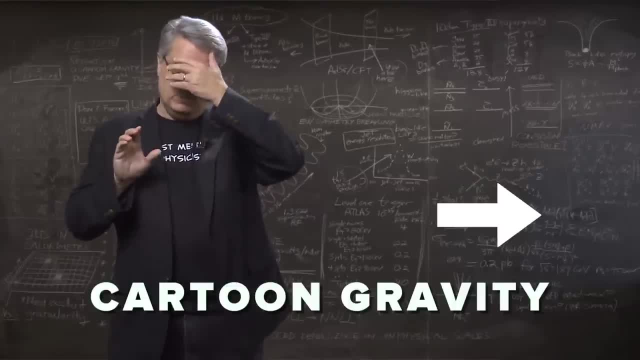 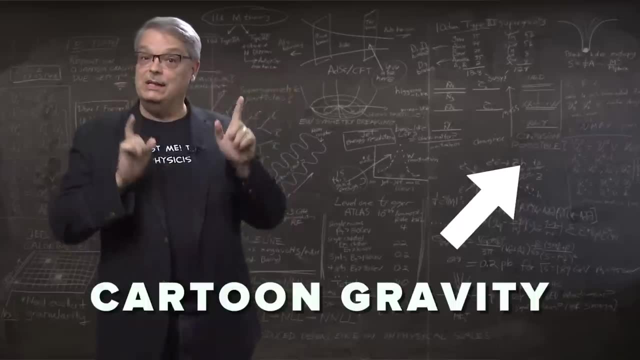 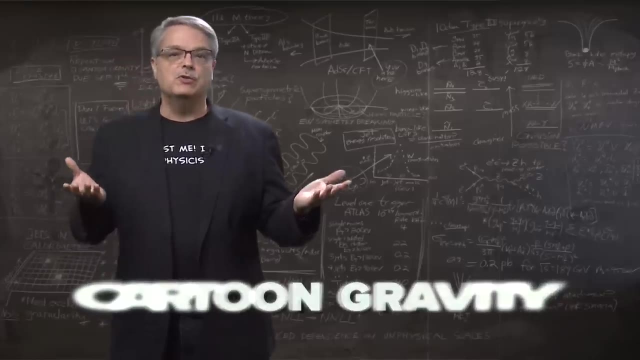 me what it is. Surprise me Now. materialize a ball in my hand When I let it go. let's see what it does. So it went that way. So that means that cartoon gravity was pointing that way. Now, cartoon gravity isn't a real thing. We can't arbitrarily point gravity. 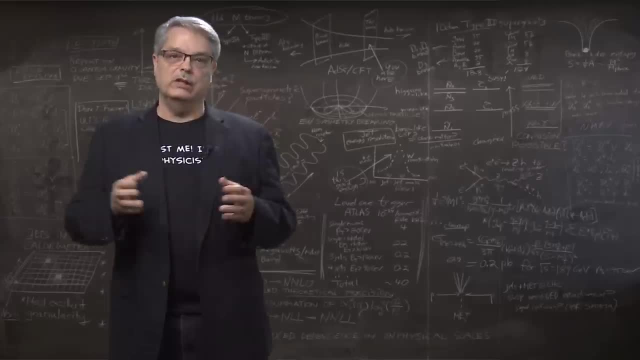 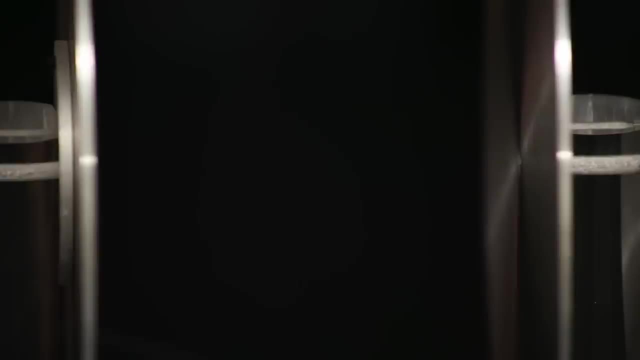 in any old direction. However, we can do that with electric fields. Let me show you how. The easiest way to make a simple electric field is to get two metal plates like these here. If we connect the two plates to the opposite sides of a battery, it will set up. 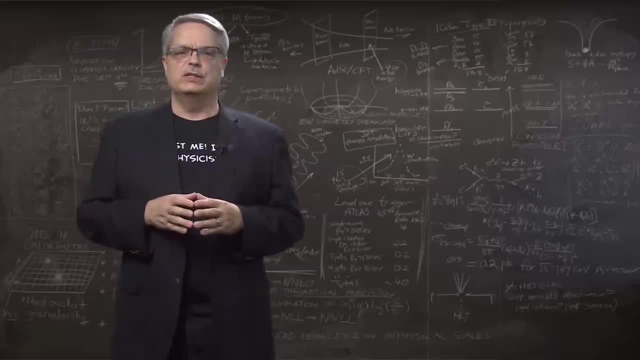 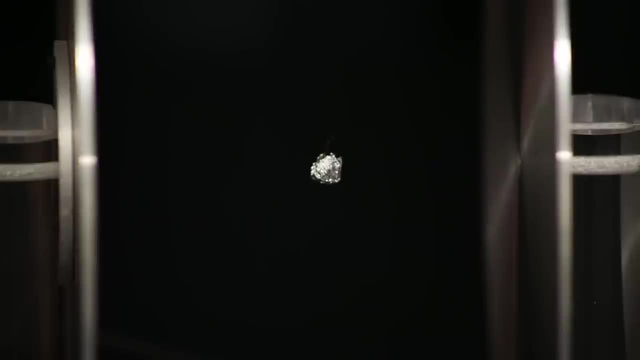 an electric field between the two plates. We won't make the connection just yet. Now we also need an electrically charged object. Okay, so now we'll connect the wires from the opposite sides of the battery to the plates and let's see what happens. So we connect the one wire. Now focus on the ball. I'll 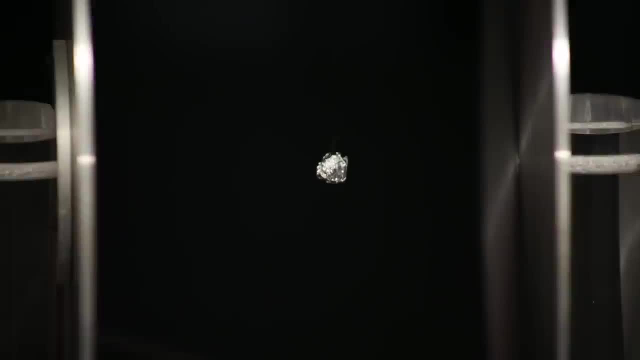 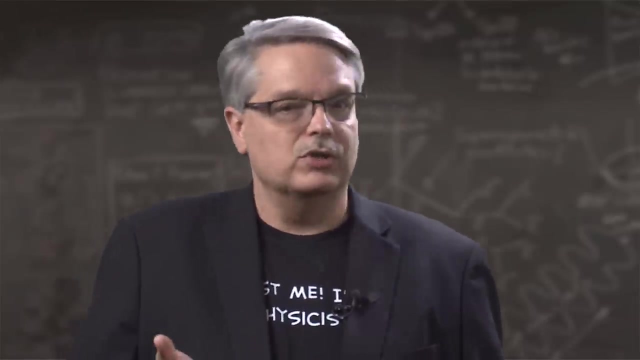 do a countdown on what happens as we connect the other wire. Five, four, three, two, one connect, Voila. The electric field makes the electric charge combine to make a force. Okay, so that's the electric field in charge. What about the circle versus line thing, Suppose? 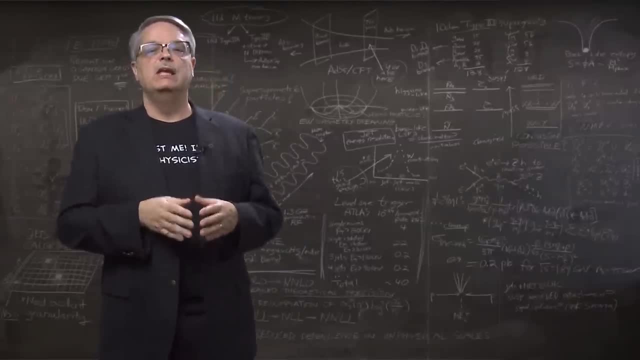 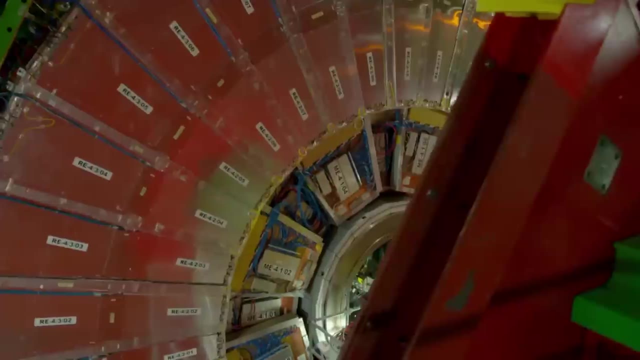 we wanted to use the very strongest electric fields possible and we wanted to make a beam of particles with the energy of the Large Hadron Collider, or LHC, which is the highest energy particle accelerator in the world. What would a straight accelerator look like? 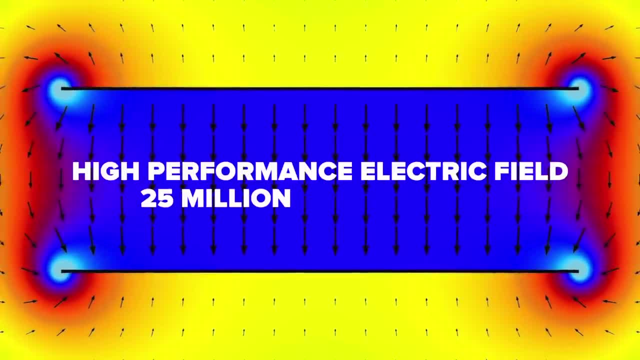 Well, a strong but technically feasible electric field might be about 25 million volts per meter, Since the LHC has a designed energy field. the LHC has a designed energy field and the LHC has a designed energy field. The LHC has a designed energy field and the LHC 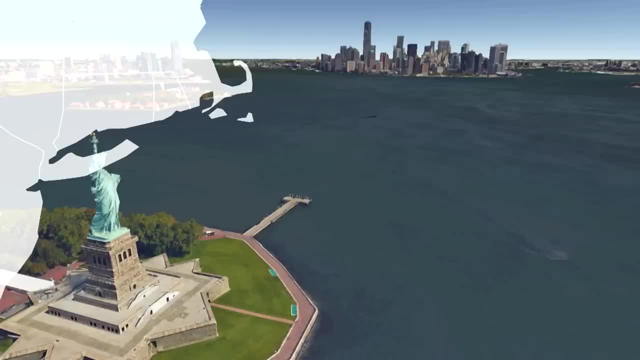 has a designed energy field. The LHC has a designed energy field and the LHC has a designed energy field. The LHC has a designed energy field. The LHC has a designed energy field. So if we wanted to use the energy of seven trillion electron volts, that would take an. 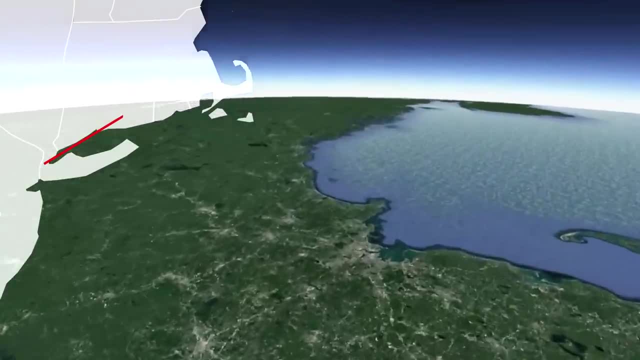 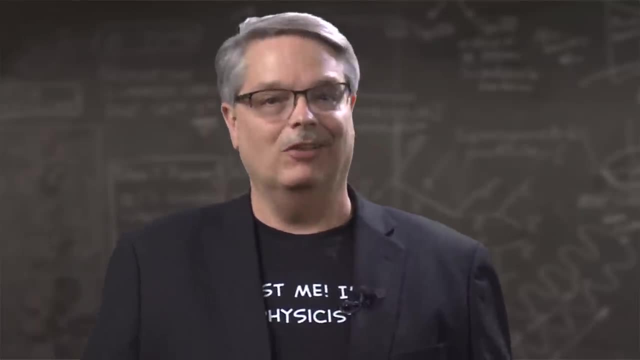 accelerator about 280 kilometers or about 170 miles. That's about from New York City to Providence, Rhode Island. So building an accelerator that long would be hugely expensive. So that's where circular accelerators come in. Circular accelerators have some elements. 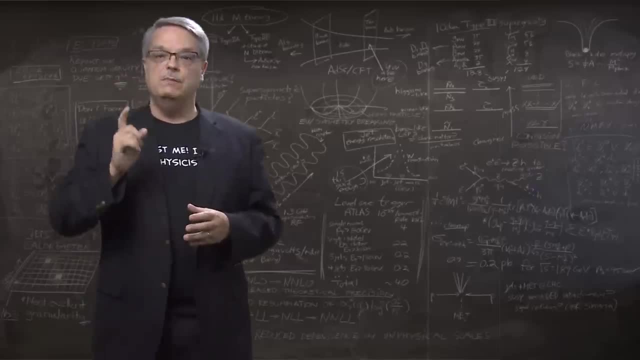 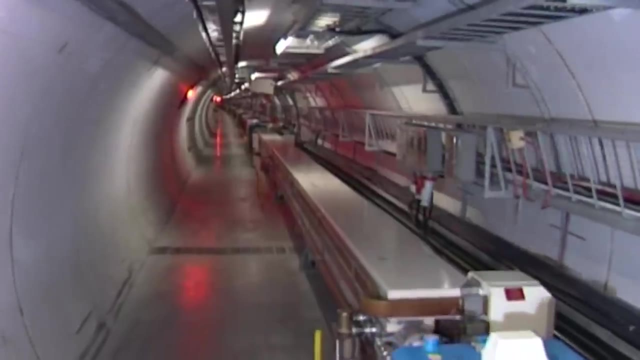 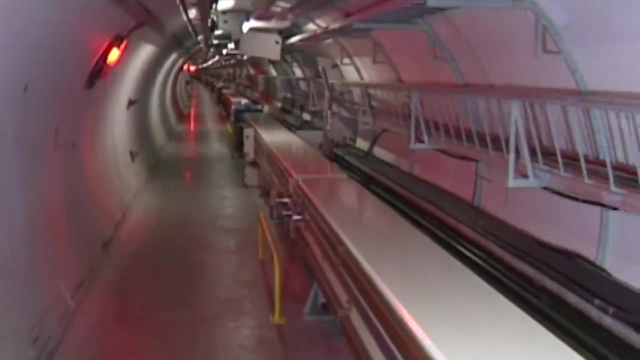 common to straight ones and some new features. To begin with, a circular accelerator doesn't have accelerators all around the circle. Instead, what they have is a relatively short length of accelerator, and the rest of the circle are a series of magnets. When a charged particle moves through a magnetic field, it moves through. 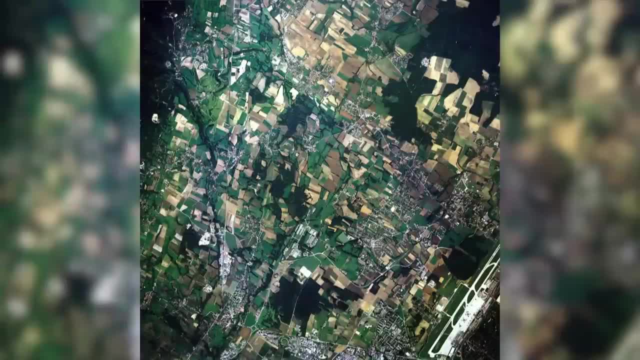 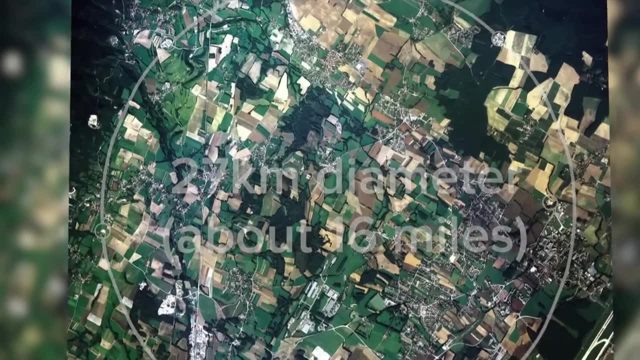 a circular path. In the case of the LHC, the whole accelerator is 27 kilometers around, or a smidge over 16 miles. But the portion of the circle that is an accelerator like we've talked about so far is just over two meters or six and a half feet Over those. 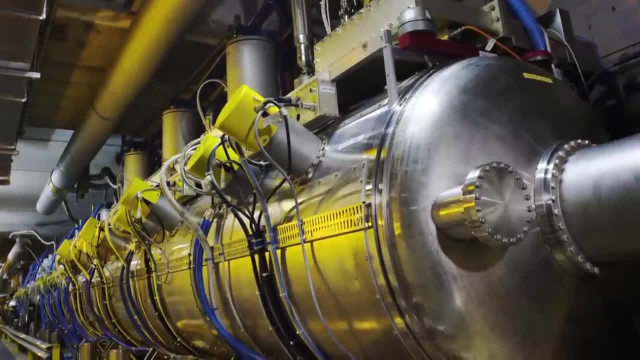 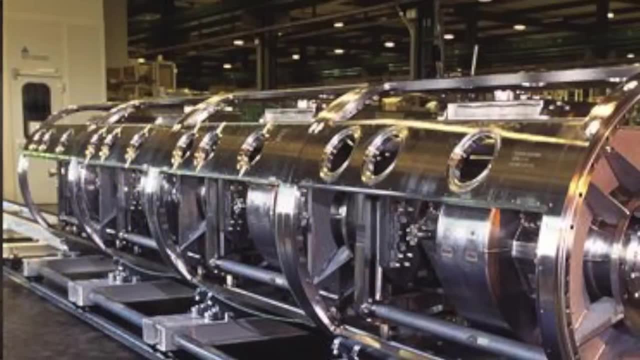 few meters. the electric field is effectively 8 million volts per meter. Although if you look it up, you'll find that the electric field is effectively 8 million volts per meter, You'll find different numbers for technical reasons. The outcome of this design means that when a proton, which is the particle, accelerated, 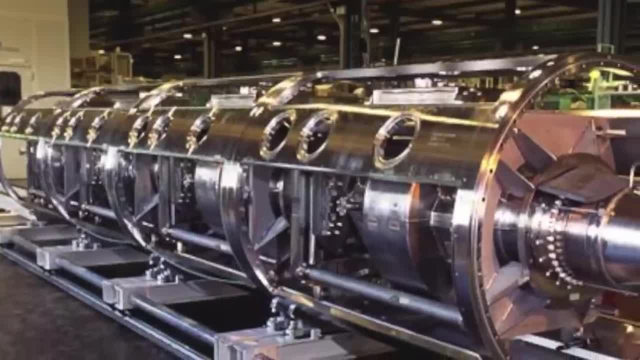 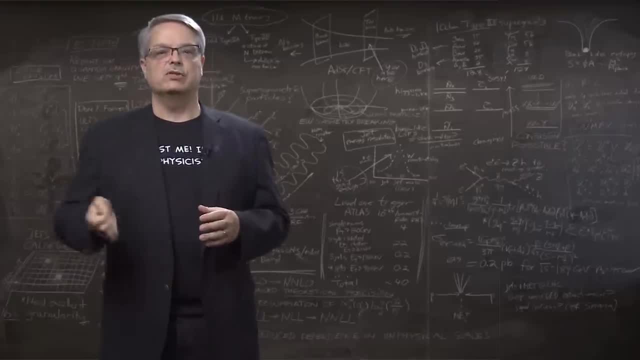 by the LHC goes through the acceleration region, its energy goes up by 16 million electron volts. With each orbit, the beam gets more and more energy, cycle after cycle. It's like a child's merry-go-round, in which an adult throws the same handle over and over again as it spins. 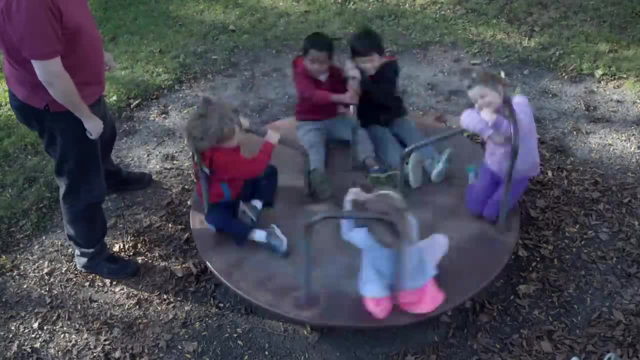 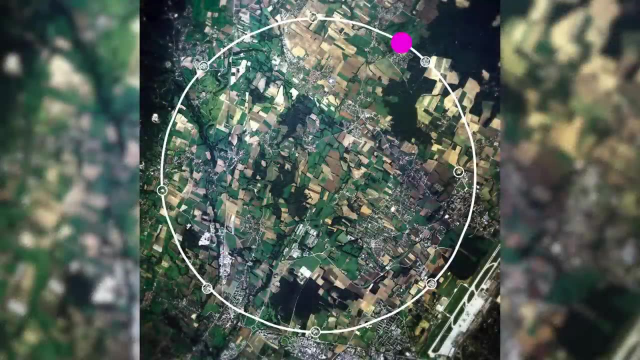 The merry-go-round goes faster and faster. Of course, if the energy is involved, the beam is already moving. The LHC is moving near the speed of light, so the beam doesn't actually speed up, But it does gain energy in the basic analogy of sound. 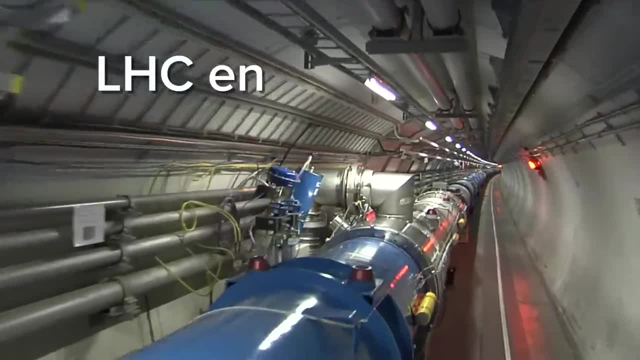 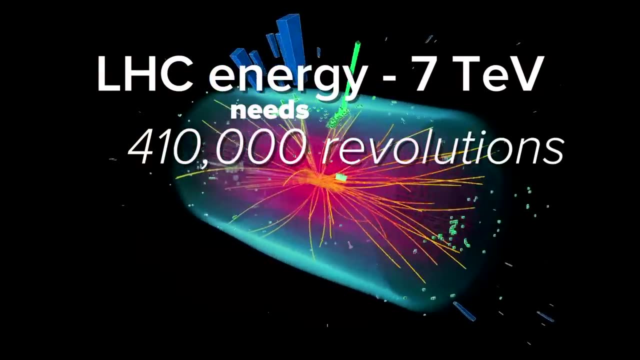 So let's think this through: To get the 7 trillion electron volt design energy of the LHC, the beam would have to go around the circle about 410,000 times. Given that the LHC beam moves at basically the speed of light, it goes around the circle about. 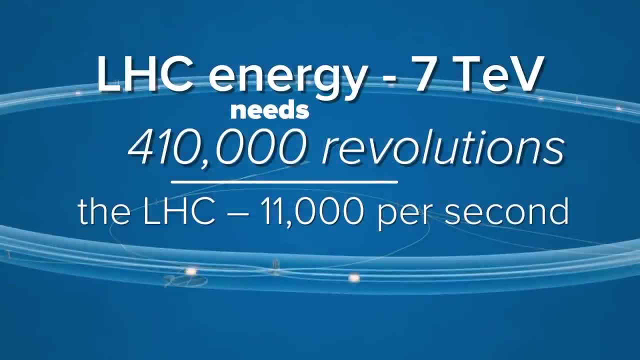 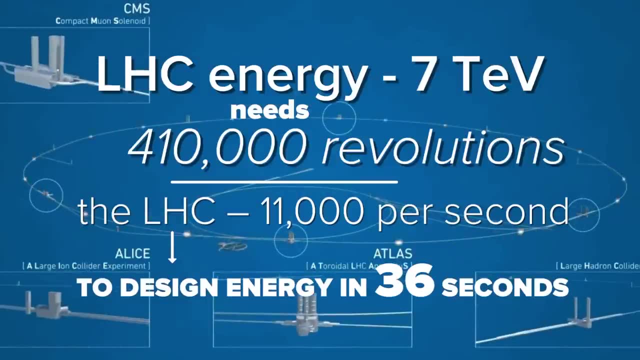 11,000 times a second. So that means the LHC could, at least in principle, accelerate a beam to design energy in 36 seconds. Now it actually takes longer than that, but that's because the energy of the beam increases. 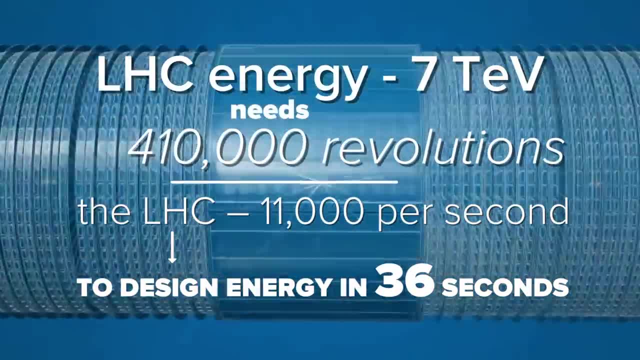 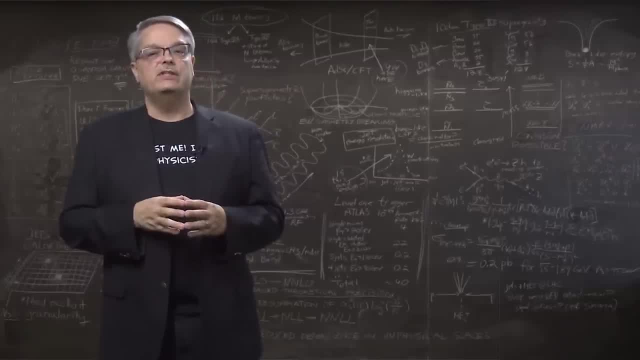 The strength of the magnet also has to increase to make the beam travel in a circle of constant radius. On the other hand, a circular accelerator is harder. In the case of the LHC, the beam goes around 11,000 times a second and the beam can circulate in the machine for 12-ish. 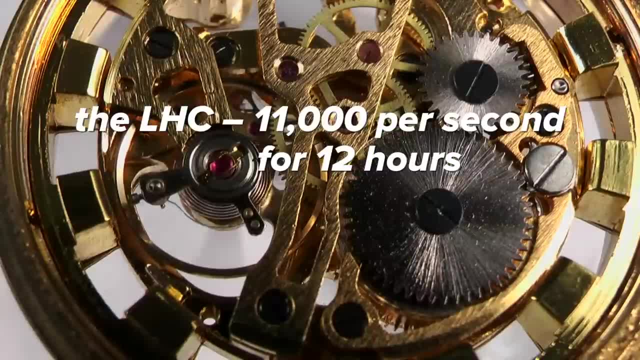 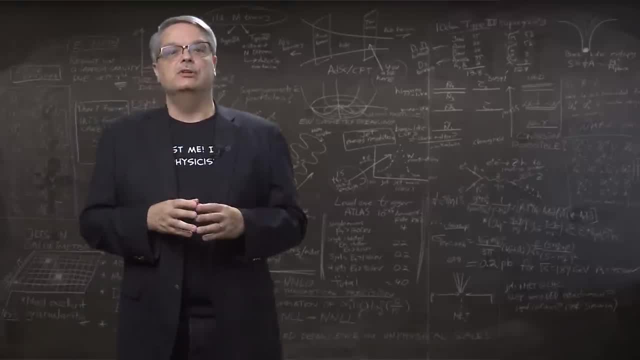 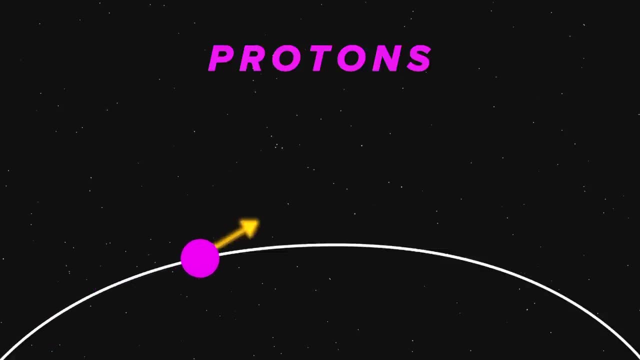 hours. That means everything has to work to incredible precision to keep the beam from inside the accelerator. So that's one minus for a circular accelerator. There's another consideration about linear versus circular accelerators. When you force an electrically charged particle to move in a circle, it gives off radiation, which makes